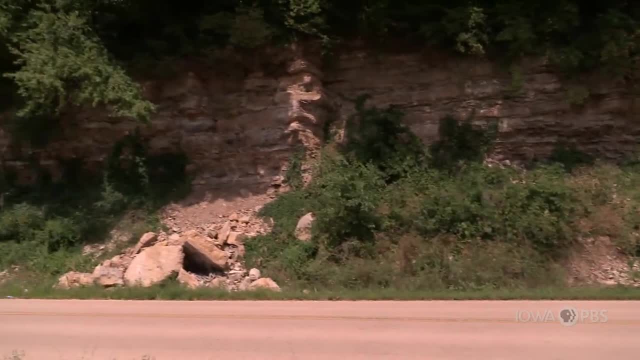 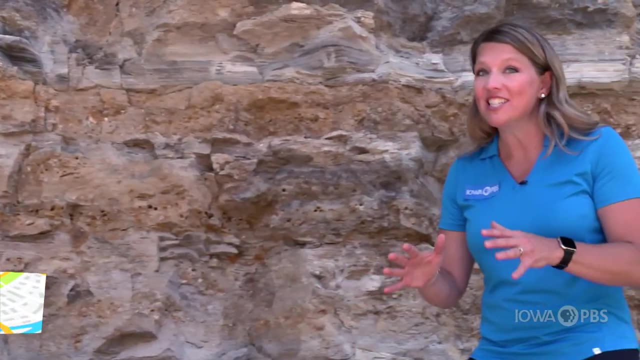 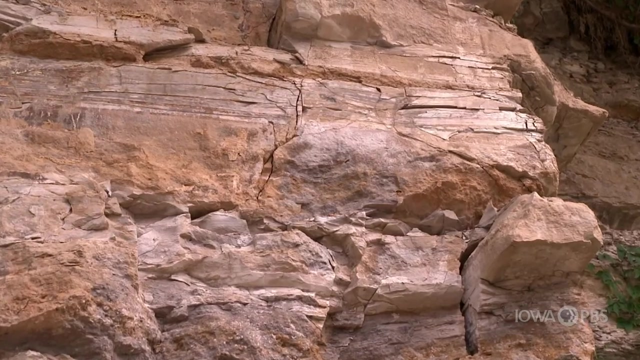 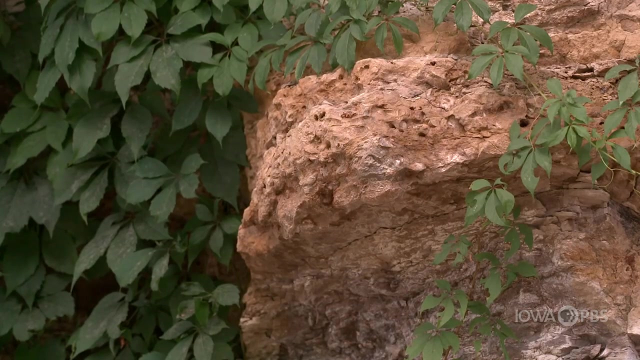 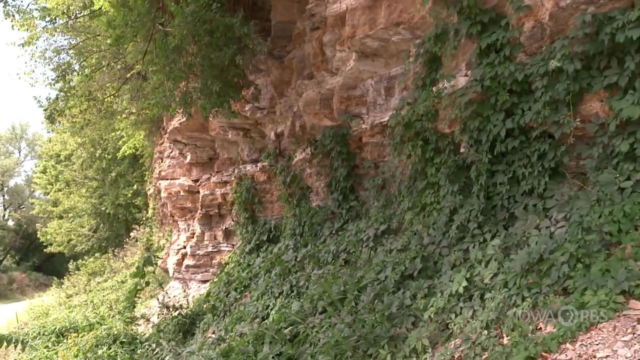 This is a very unique spot in Iowa where we can learn lots about our geological history by studying the changes in the layers of this rock. Where could I be in Iowa? Come explore with me. Sometimes the rocks that tell the history of Iowa are in places where people drive by every day without ever recognizing how special they really are. 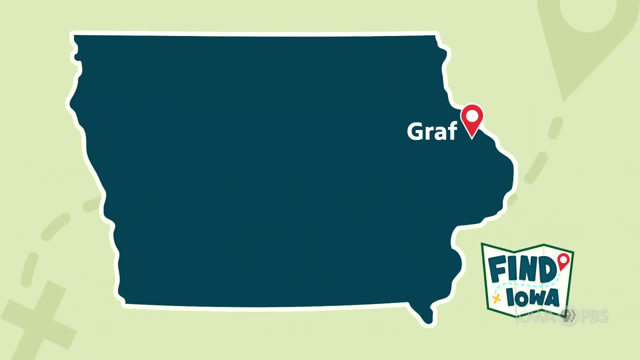 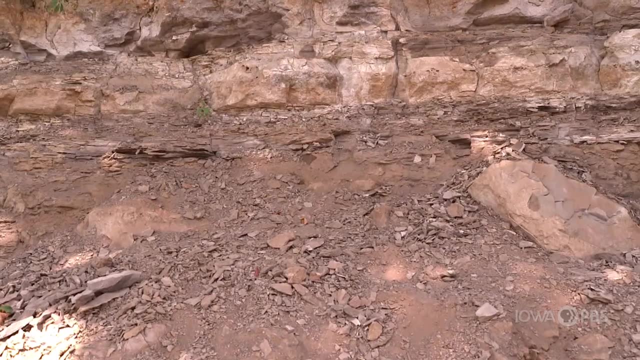 Just like the rocks we're exploring today in northeast Iowa, in a town called Graff, where we can see layers and layers of ancient rocks right on the side of the road By studying the layers from the bottom all the way up to the top. 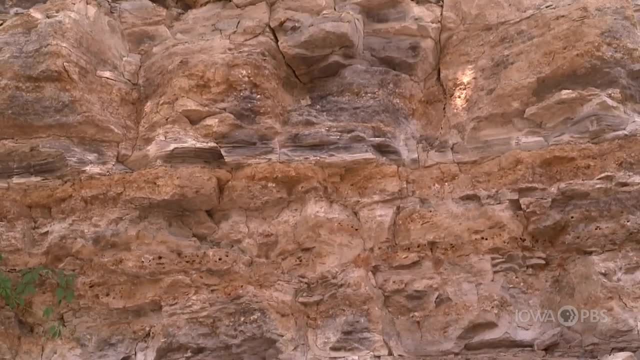 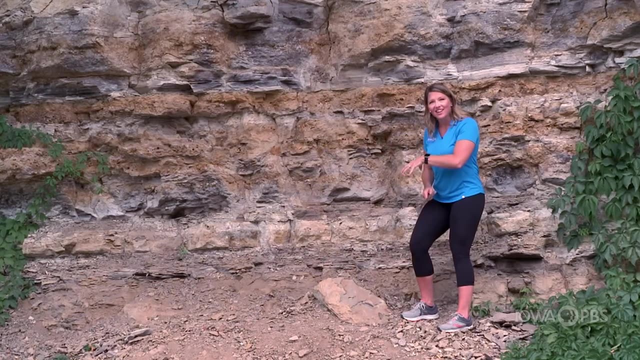 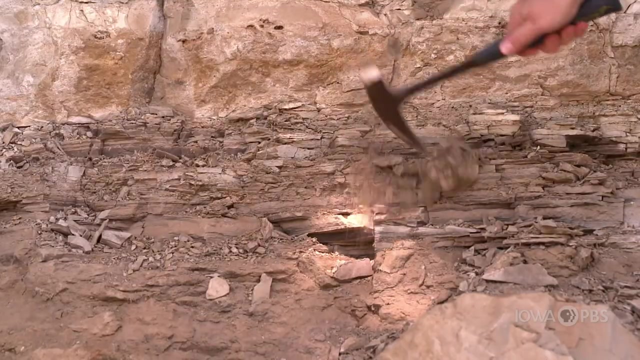 we can tell so much about Iowa, Let's explore Iowa's history. Millions and millions of years ago, this rock was deposited in Iowa. My good friend, John lent me one of his favorite geology tools to take a closer look. Some of the layers are made out of shale. 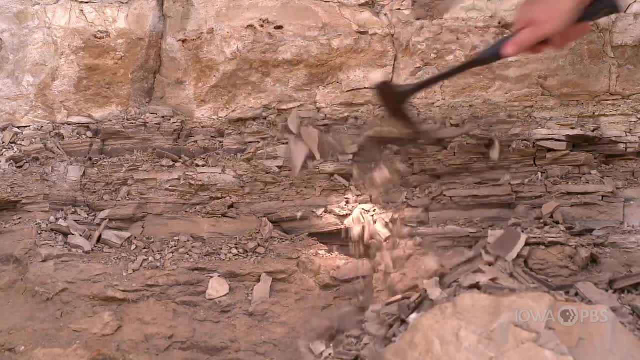 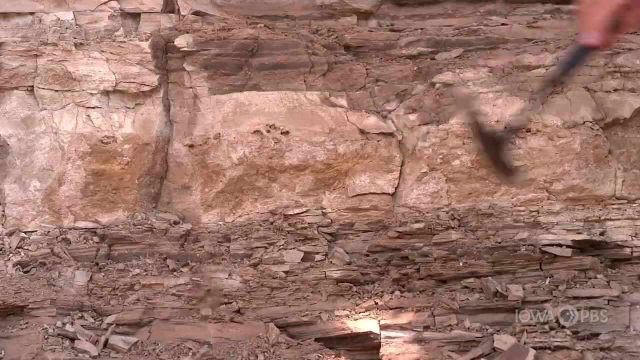 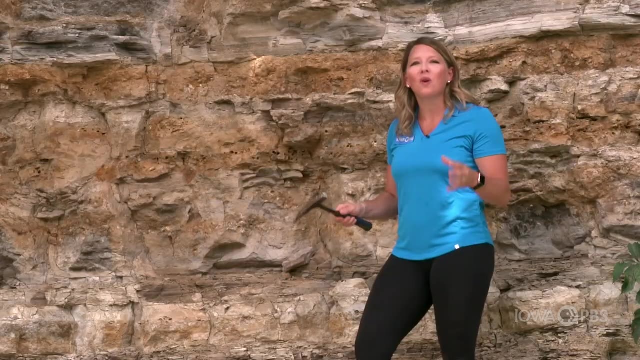 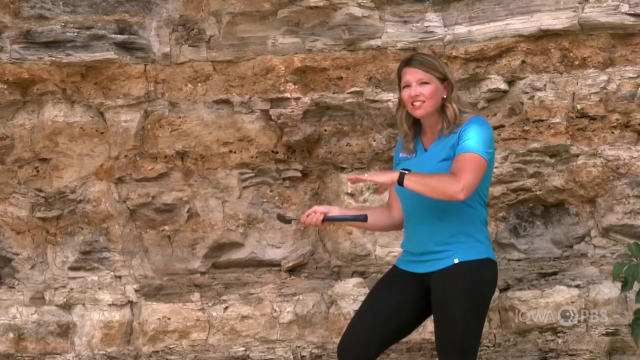 They're softer because they're made out of clay and sand. Some of the layers are made out of limestone. They're a whole lot harder. These layers of limestone and shale are evidence that Iowa was once covered in a warm tropical sea. The alternating layers tell us that the sea sort of came and went. 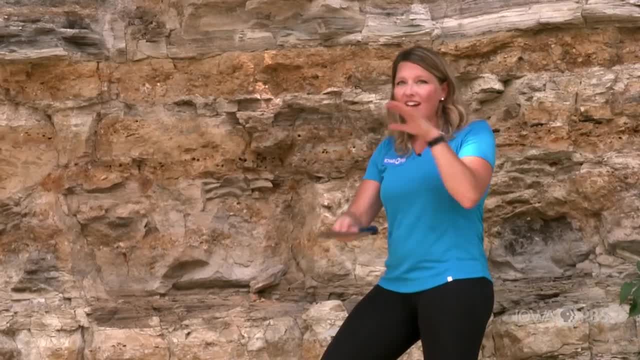 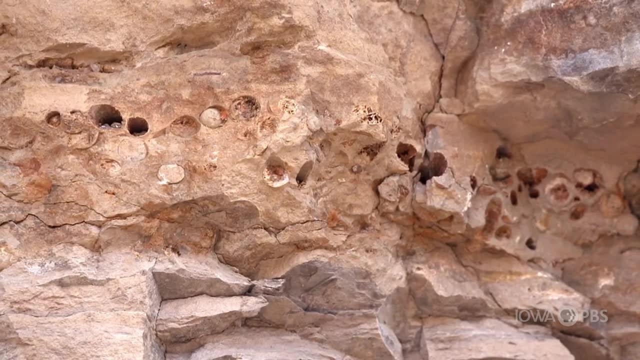 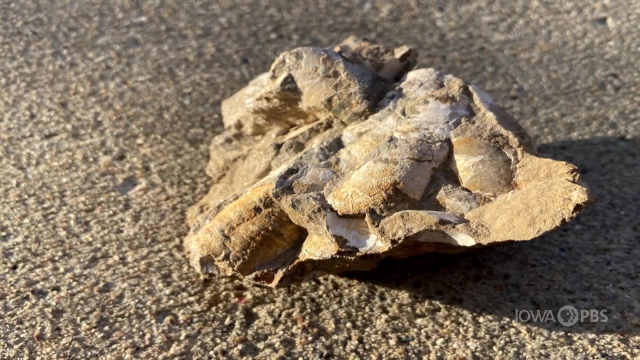 Or there were times where it was much deeper and much shallower. The limestone contains even more evidence of Iowa's history. Can you guess what it is? The limestone in Graff Iowa is so deep that it's hard to believe. The limestone in Graff Iowa is so special because it contains fossils. 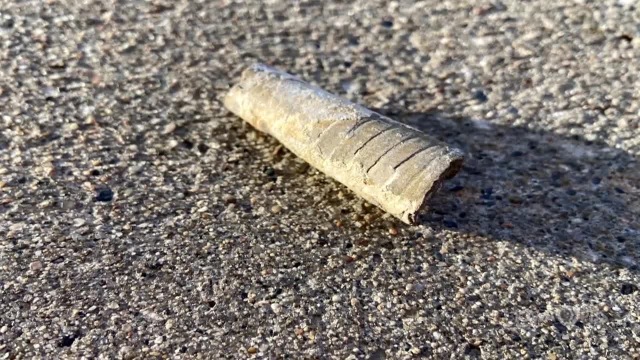 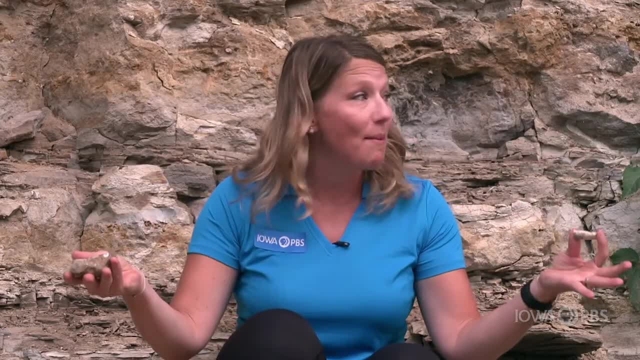 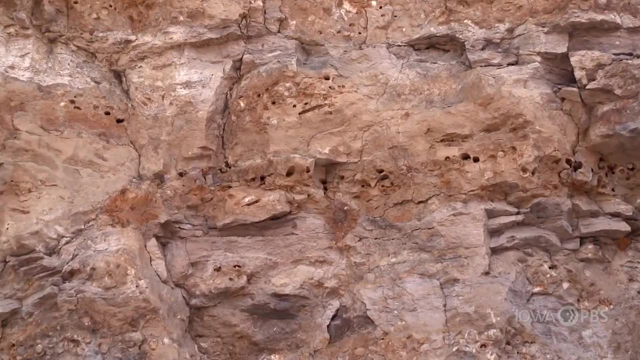 These fossils are actually sea creatures. This fossil is a nautiloid cephalopod. These creatures lived in the warm tropical sea that once covered Iowa. So how does a creature once living and swimming around in the sea become fossilized and part of a rock?